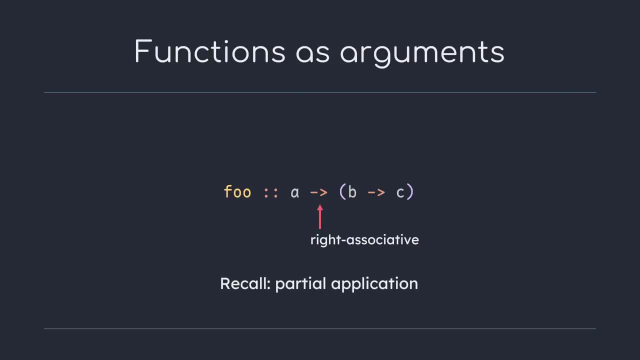 So in order to define function arguments in our type, we write a function within parentheses. This would be a function that takes a function a to b as an input and returns a value c. Functions like this, that take other functions as arguments, are called higher order functions. 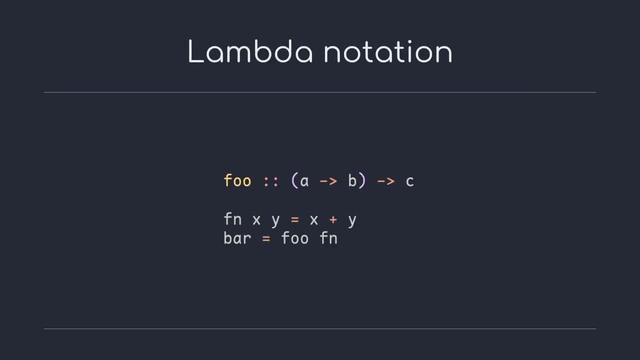 When feeding a function into another function, we can use name functions, but sometimes it is more convenient to inline the function definition somehow. Haskell makes this possible with what is called lambda notation. This code yields an anomalous function that adds two numbers, x and y. 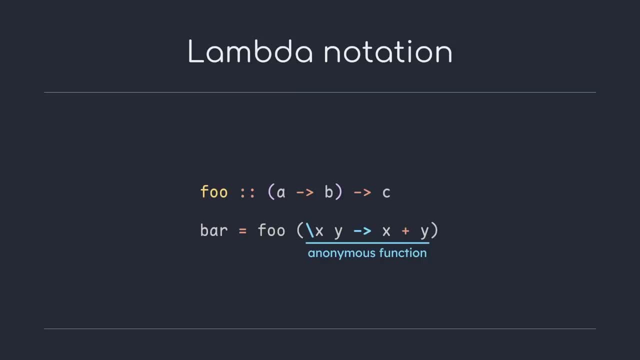 And this way we can inline the function definitions into arguments of other functions. A common pattern when working with lists is applying a function to every element in a list. Think of formatting a list of numbers to display them, or just updating a list of objects according. 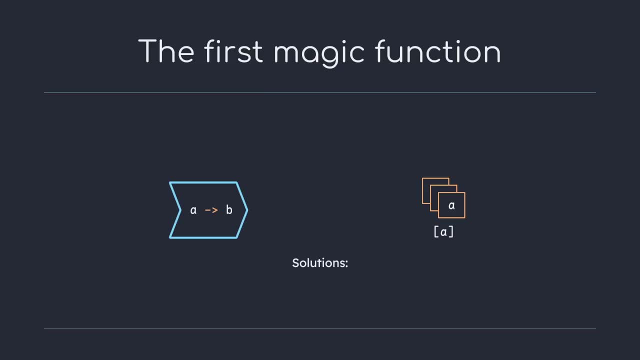 to some update function. We already talked about list comprehensions and how these perform. We can provide a shorthand way of achieving this behavior without resorting to trivial recursion every time. However, there is an even shorter way to implement this behavior using a function with function. 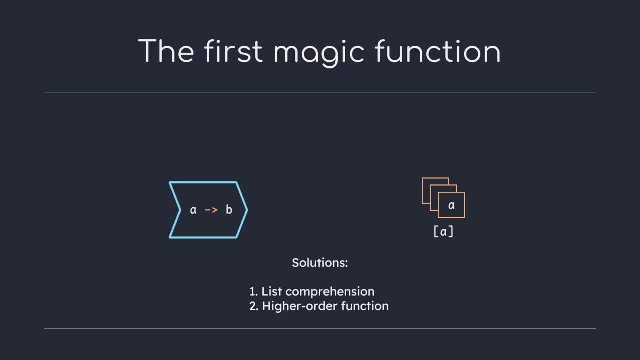 arguments. The best way to understand most Haskell functions is to make them ourselves, so recall Hutton's method from last video. Let's call our function apply for now, And it should take a unary function. a to b, a list of elements of type a and when each. 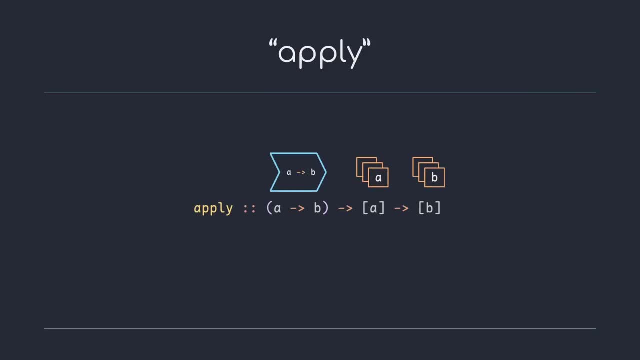 of these elements gets passed into the function, it becomes one of type b. So a return type will be a list of elements of type b. Now the definition of the function we are passing in stays the same throughout the entire recursion tree, so we only need two cases for our list. 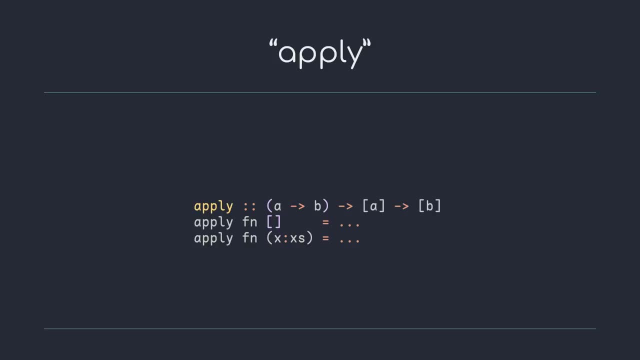 And for lists, the cases are as follows: Defining the cases, the return type is going to be a list, so our base case should return empty list and our recursive case should return a const. And it should then make sense that applying fn to x and applying apply with fn to the 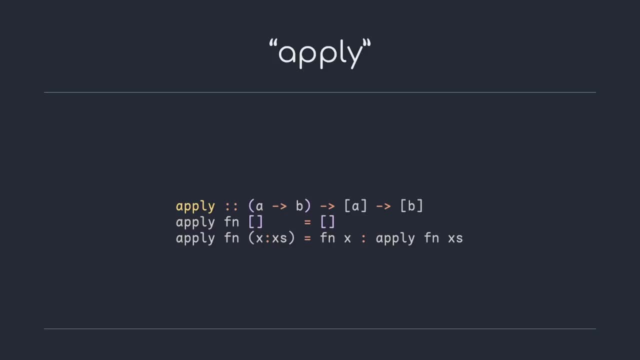 remaining x's gives us the desired behavior. This function already exists in the standard library of Haskell. It is called map and it is one of the most important and commonly used functions in the entire language. And this is because map solves a problem that is very common: mapping a function onto a. 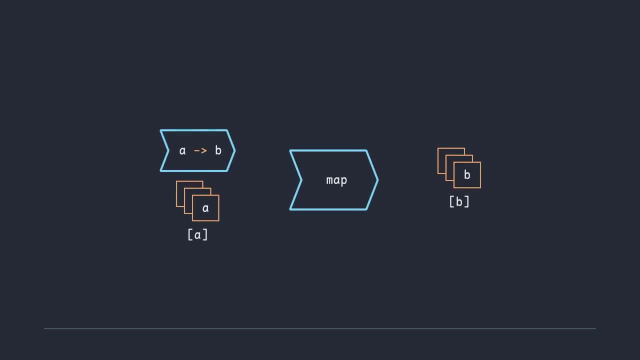 list. Another way to think about map is to partially apply it. If we only feed a function into map, The resulting type will be list of a to list of b. So in a way, map creates this function on list from a function on elements. 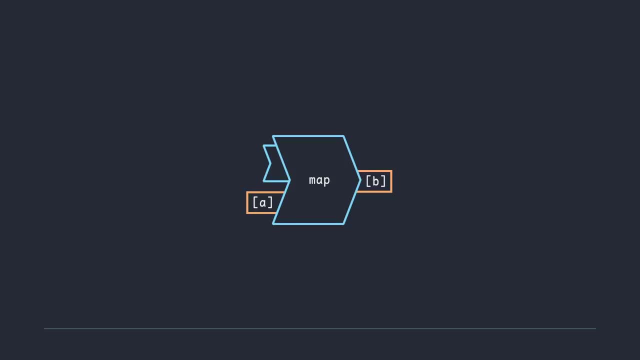 And this is noteworthy because it allows us to start thinking about functions like building blocks rather than actions or operations. Large functions become more like machines made out of smaller functions, which are like lego bricks. We will explore this idea of thinking about functions further in an upcoming video. 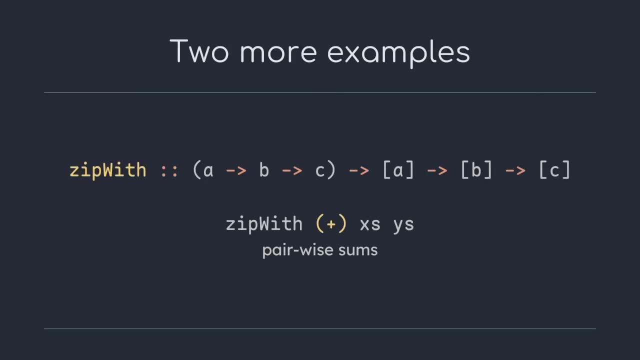 For now let's look at two more examples. ZipWith takes two lists and combines the corresponding elements using a binary function. So zipWith plus x's, y's will give the pairwise sum of x's and y's. Its cousin, zip, combines the elements into tuple pairs. 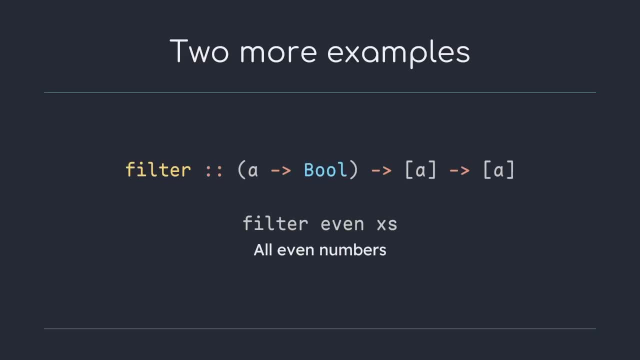 Filter takes a list and returns all the elements where the given function returns true for that element. So filter even x's returns all the even numbers in x's. ZipWith takes two lists and combines the corresponding elements using a binary function. So filter even x's returns all the even numbers in x's. 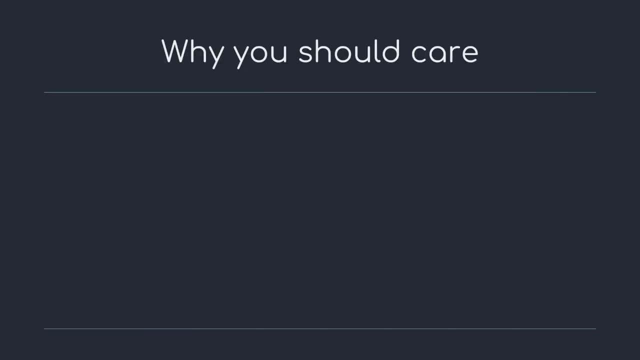 So why is this so important? First and foremost, knowing that these functions exist and are probably already written for you by someone else means you can drastically increase your productivity. Maps solves a very simple problem in our case, but a more complex pattern like fold or scan. 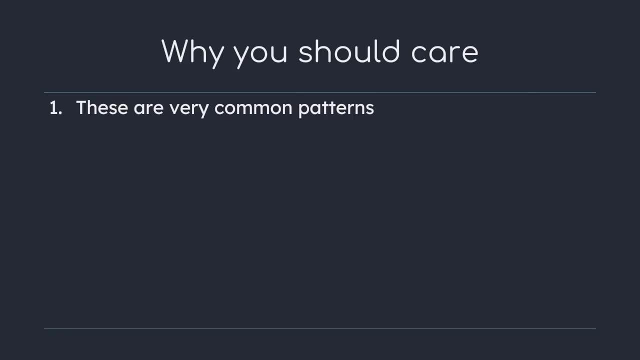 can save you a lot of time. In some cases, this can even improve performance. Since these functions are so general purpose, there's a good chance that their implementations are already heavily optimized. For example, the problem that map solves is embarrassingly parallel, and filter can be. 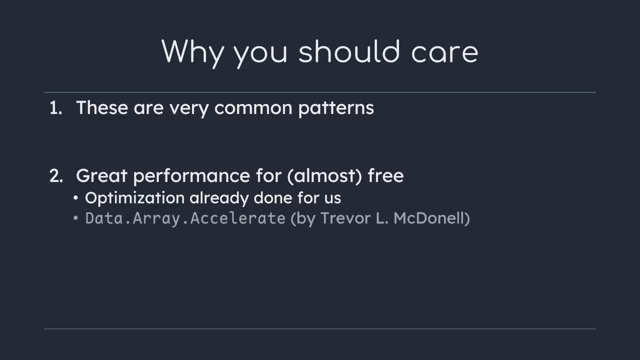 implemented using a divide and conquer strategy And indeed people already have written these standard library functions with things like hardware acceleration. In fact, the person who wrote this library was also my professor in concurrency and parallelism. Of course, case-specific optimizations are not taken into consideration with this approach.